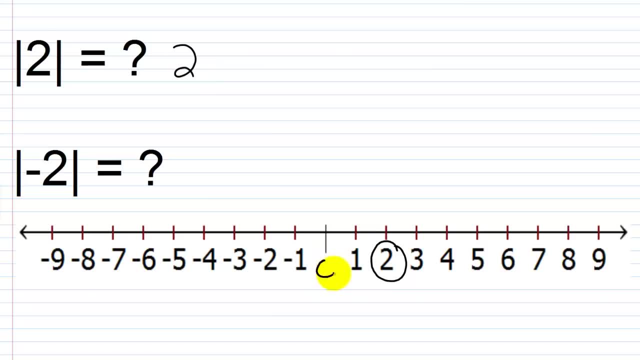 on your number line. Look at 2 on your number line. Look at 2 on your number line. Look at 2 on your number line. 2 is right here, 0 is right here And 2 is 1, 2 units away from 0. And it. 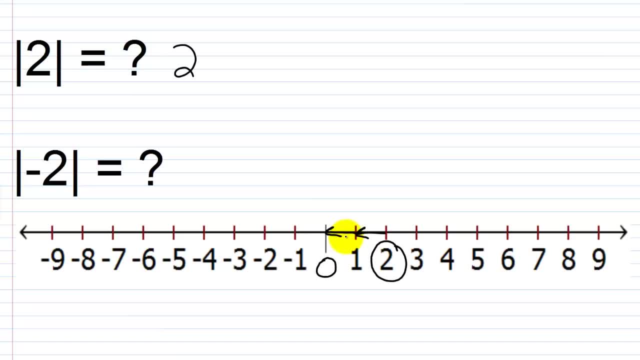 doesn't matter the direction you have to move to get to 0. It's just in terms of how far do I have to move? So it's 2 units away from 0. So the absolute value of 2 is 2.. Now also negative 2. 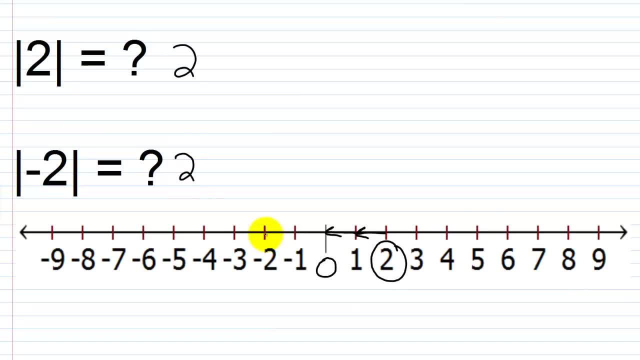 has an absolute value of 2, because you have to move 2 units to get from negative 2 to 0 as well. So look you go 1,, 2 units that way to get to 0. So two numbers with the same absolute value. 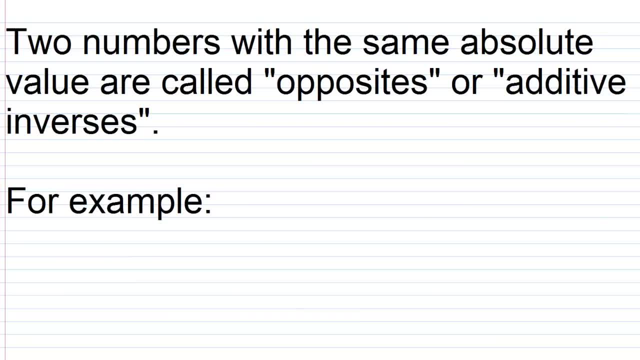 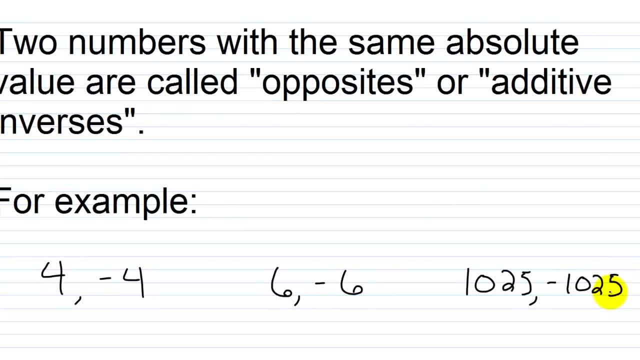 down a little bit. Okay, those would all be opposites And, as we just saw, each would have the same absolute value. So 4 and negative 4 would have an absolute value of 4.. 6 and negative 6 would have an absolute value of 6.. And 1,025 and negative 1,025 would have an absolute value of. 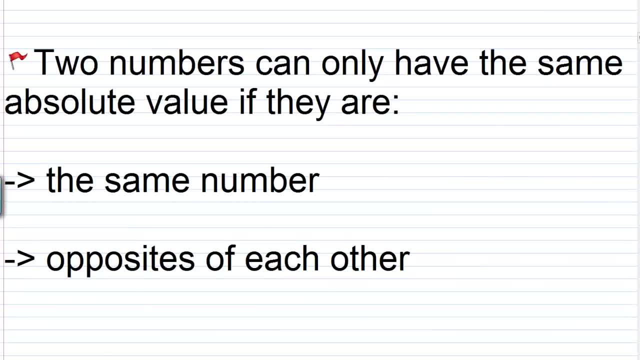 1,025.. And just one more quick point before we get into actually solving equations: Two numbers can only have the same absolute value if they are the same number. so obviously if you have the same number, like 2 and 2, right, that's going to have the same. 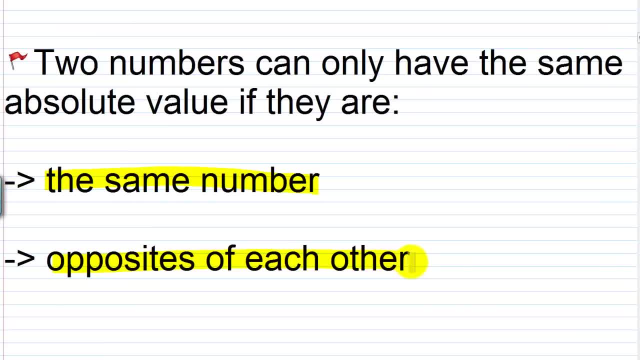 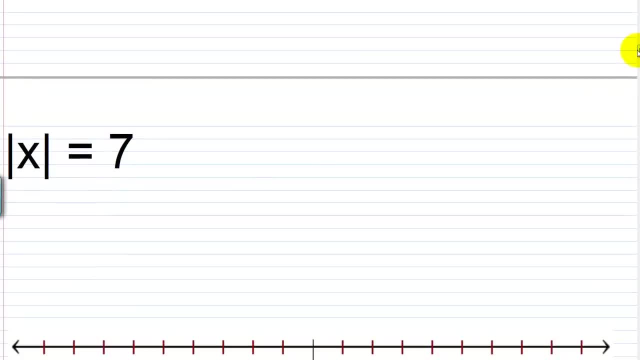 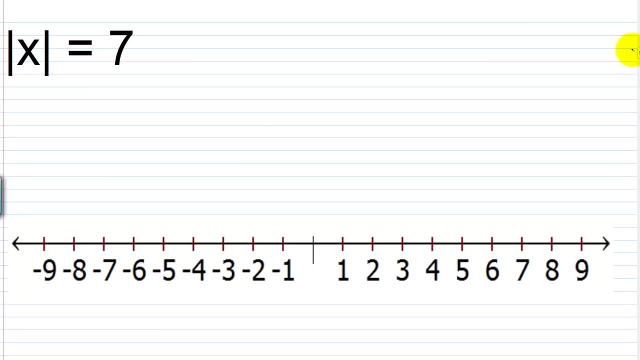 absolute value And then opposites of each other. okay, opposites of each other. So 2 and negative 2 would have the same absolute value. Let's look at something easy to get started. Let's say we have the absolute value of x equals 7.. So what am I asking for here? I'm asking for what numbers? 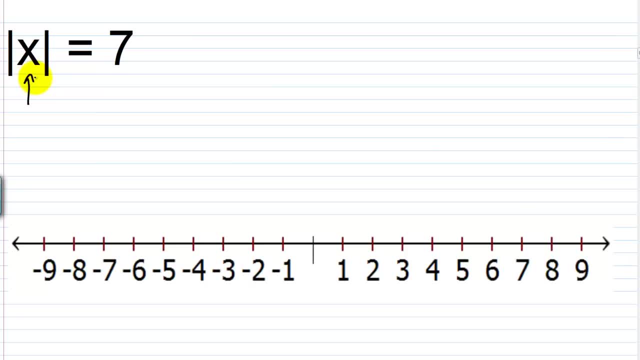 can I plug in for x there and get a true statement. So plug something in for x, take the absolute value of x and plug it in for x, And then what am I asking for here? I'm asking for what numbers can I plug in for x, take the absolute value of it and get a 7.. So what two numbers do we know of? 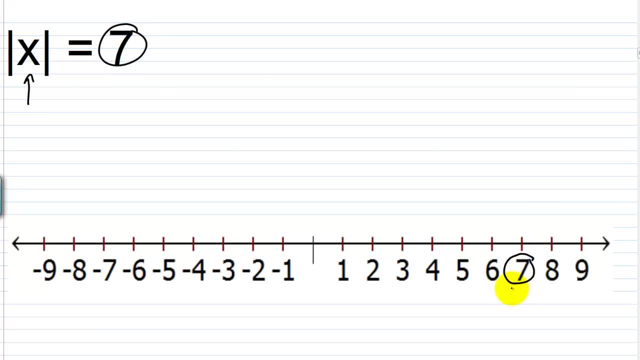 that have an absolute value of 7? Where there's 7 and there's negative 7.. Each is 7 units away from 0 in the number line. So when you see something like this, basically you're going to think about just saying that x could be equal to what, It could be equal to 7, or it could be. 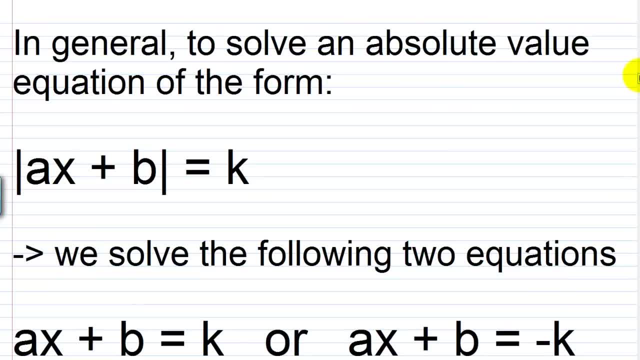 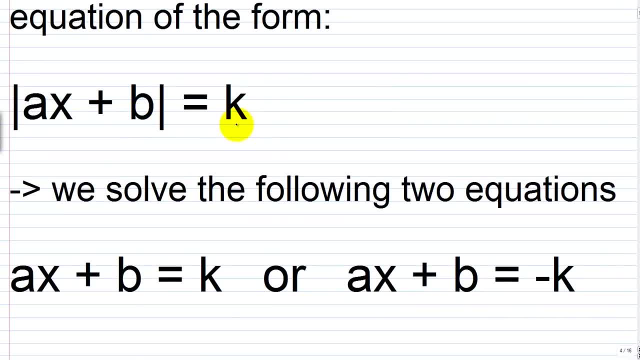 equal to the negative of 7.. Okay, so in general, to solve an absolute value equation of the form, here we have the absolute value of ax plus b equals k. we solve the following two equations: Ax plus b could be equal to k, right Positive k, Or ax plus b could be equal to the negative of k. 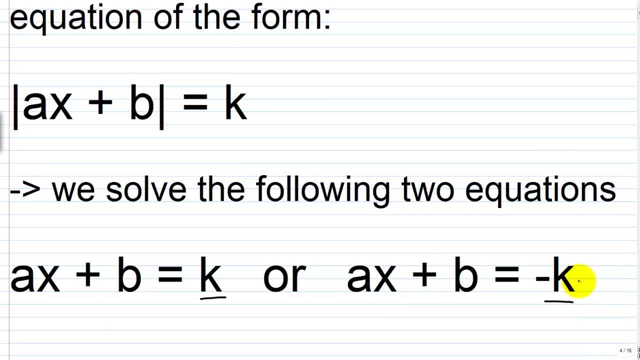 Because if we take the absolute value, okay, it's going to end up being positive Okay. So in other words, if this ends up being equal to negative k, once we take the absolute value of it it ends up being positive k. And I know when we start working with kind of abstract stuff it gets confusing. 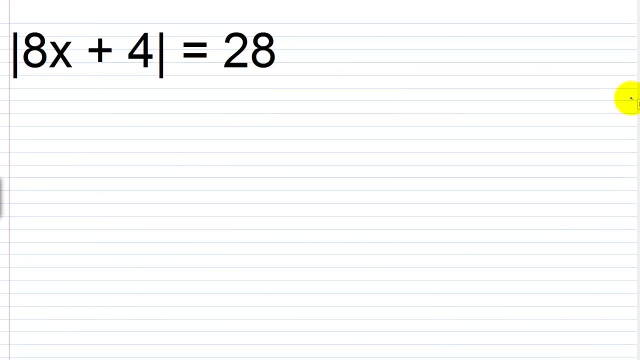 but let's jump in and look at an example. So we have the absolute value of 8x plus 4 equals 28.. So following that rule, we would set up these two equations: 8x plus 4 could be equal to 28,, or? 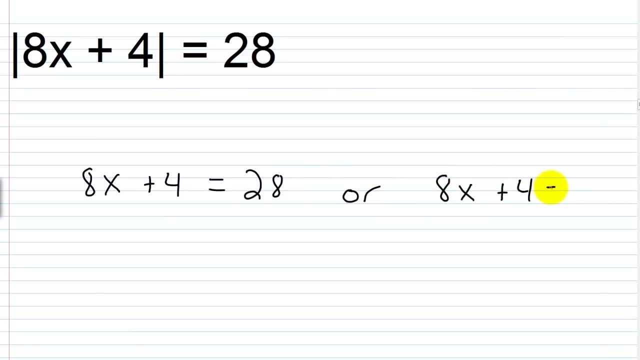 8x plus 4 could be equal to negative 28.. Okay, you're going to solve those two equations. Having a hard time fitting that on the screen, Let me kind of scroll this over a little bit. And again, if 8x plus 4 was, 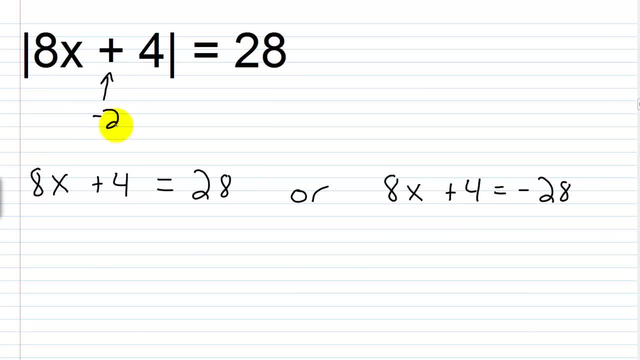 equal to negative 28,. meaning I got a value here of negative 28.. All right, I plugged in some number for x, I multiplied it by 8, I added 4 to it and I got negative 28 as a result. Once I take the 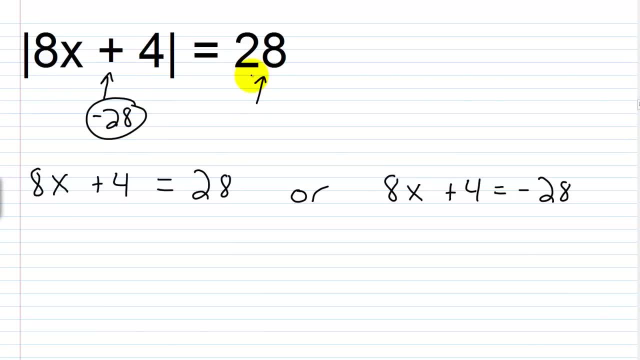 absolute value of it, I'll have a true statement, because it will be equal to positive 28.. Okay, that's what absolute value does. It takes a negative number, it makes it positive. All right, so let's solve these two simple equations. We will subtract 4 away from each. 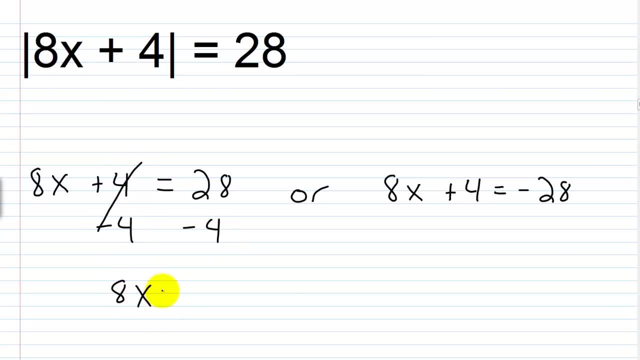 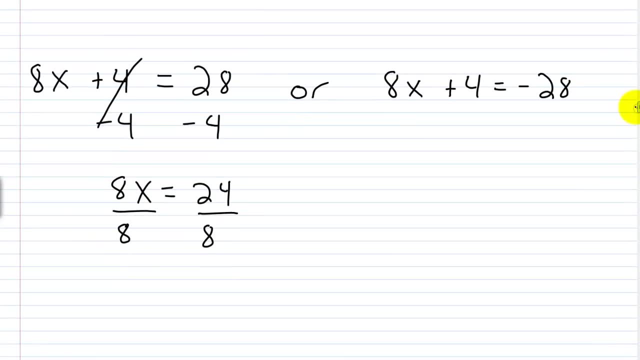 side here That will go away. I'll have 8x is equal to 24.. I'll divide each side by 8, and we'll have x equals 3.. x equals 3, so that's one solution. Okay, and then we have this, or Now I'm going to subtract 4 away from each side. here I'll 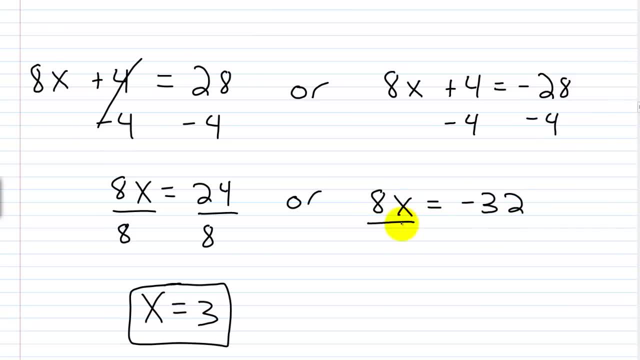 have 8x is equal to negative 32.. I'll divide each side by 8.. That will cancel with that And I'll have x equals negative 4 as another solution. So my solution set here. I'm going to provide a way for you to take a look at how you can roughly calculate a set of numbers. 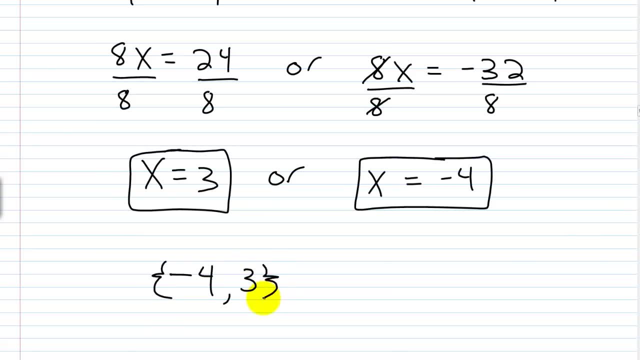 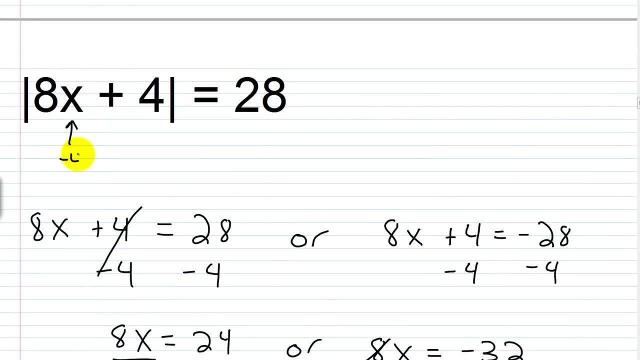 that will help you on this problem. All right, so our first-ever goal here is to find x, and the first-ever goal in this problem is to find the total value of x. The next thing we're going to do is the following. So my first-ever goal is to find the total. 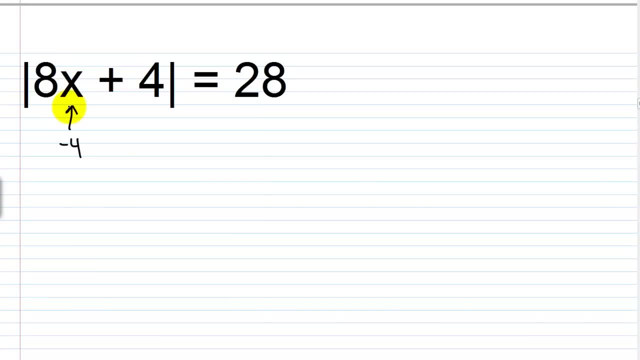 value of x. So I'm going to take my first-ever goal And I'm going to use this. Let's see. Let's see what I can do with this. So we're going to take a set of numbers. So I'm going to take a set. 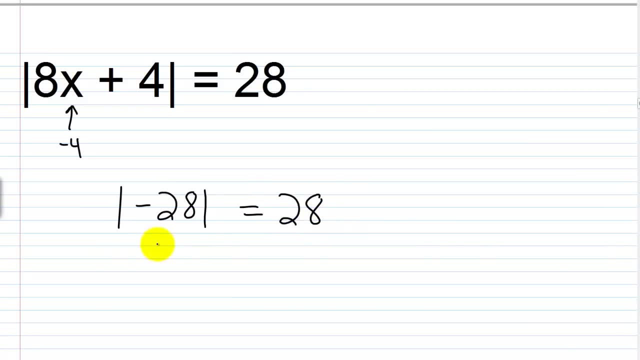 Then I'm going to multiply this by 8.. I'm going to multiply this by 8.. equals 28.. And, of course, as I explained earlier, you take the absolute value of negative 28,. you get 28.. So 28 equals 28. And we have a true statement right. So x equals negative 4. 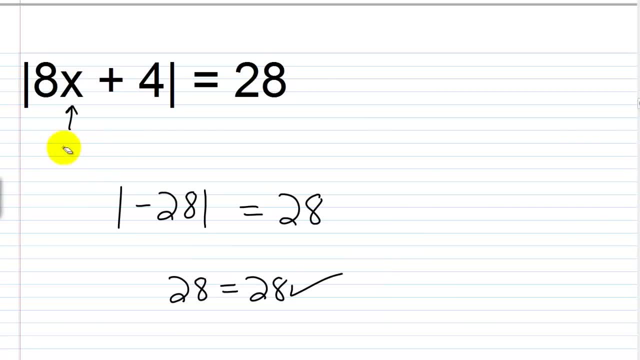 is one of our solutions. All right, so let's check: x equals 3. And basically I think you can kind of eyeball that and see it would work right: 8 times 3 is 24. Then you'd add 4, you get. 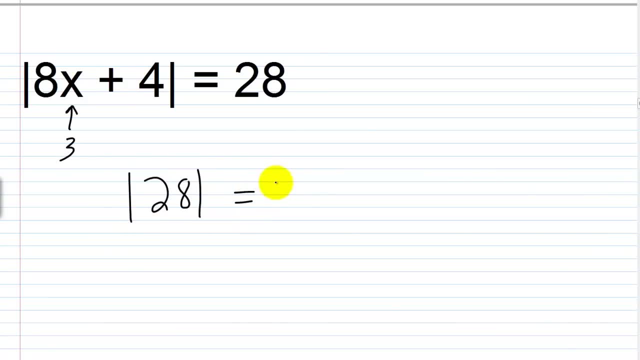 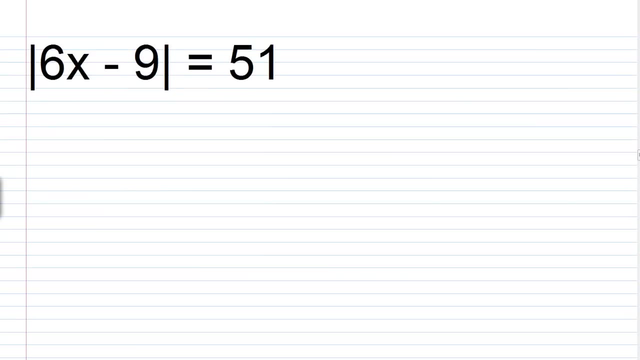 28.. So you'd have: the absolute value of 28 is equal to 28.. And of course, that's true as well. Let's take a look at a number. Okay, so we have: the absolute value of 6x minus 9 equals 51.. 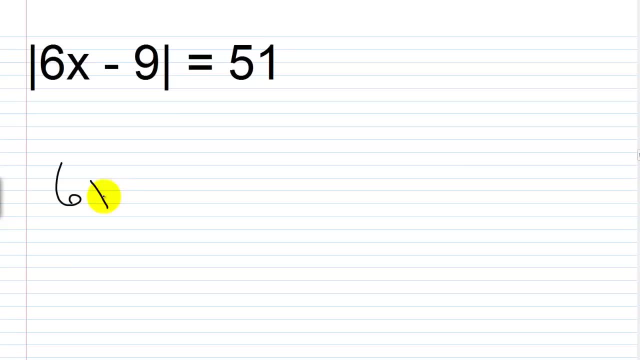 And again we want to set up two equations here. We want 6x minus 9 is equal to 51. Or we want 6x minus 9 is equal to negative 51. Because again, if I plug in something for x, 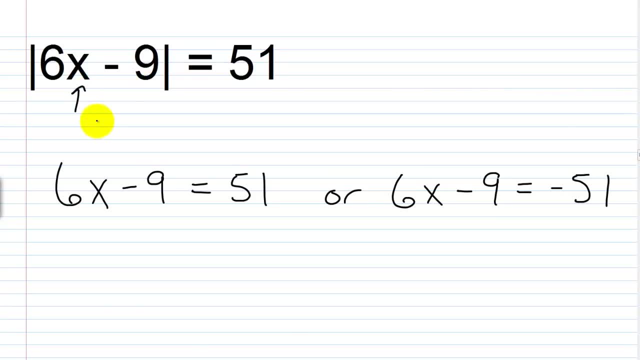 I multiply it by 6,, I subtract away 9, and that gives me negative 51. Once I take the actual value of 6x minus 9,, I get the absolute value of 6x minus 9.. And again we want to set. 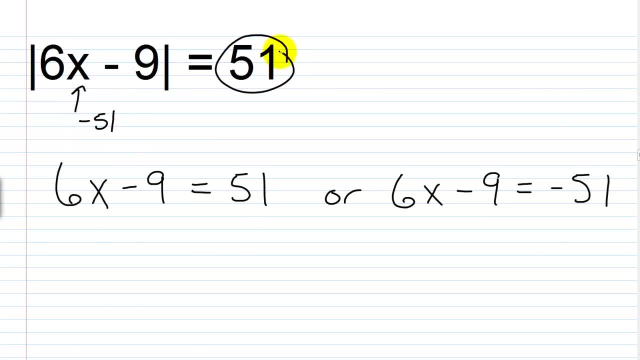 up two equations here. We want 6x minus 9 is equal to 51. Or we want 6x minus 9 is equal to negative 51. And value of negative 51, it will give me 51, so either of these would work all right. 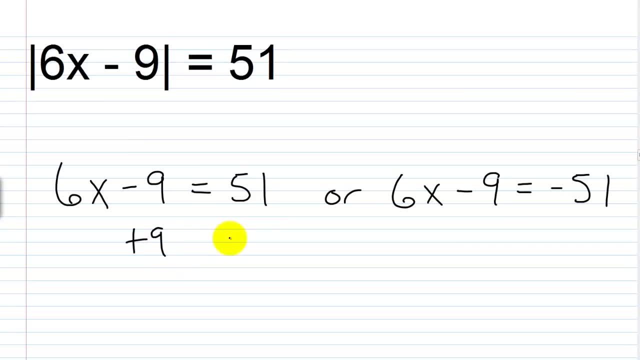 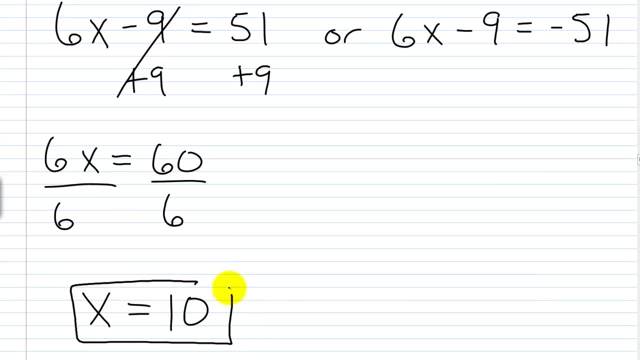 so let's solve each equation. so let me add 9 to each side that will go away. I'll have: 6x is equal to 60. of course, we all know that that's gonna be X equals 10. I'll just divide each side by 6: X equals 10. so that's one solution. let's. 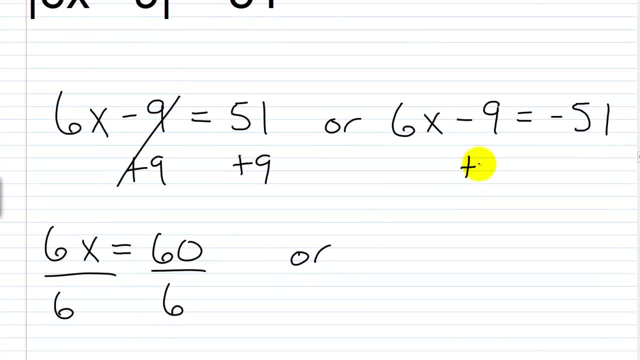 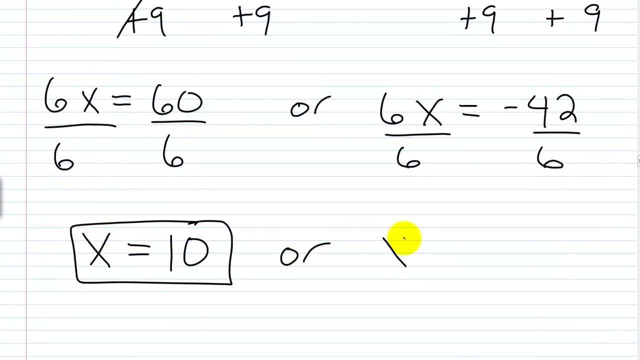 kind of come back up here, so we have this poor. let me add 9 to each side over here, so we'll have: 6x is equal to negative 42, and we'll divide each side by 6, by 6 over here, and what we're gonna get is X is equal to negative 7, so we 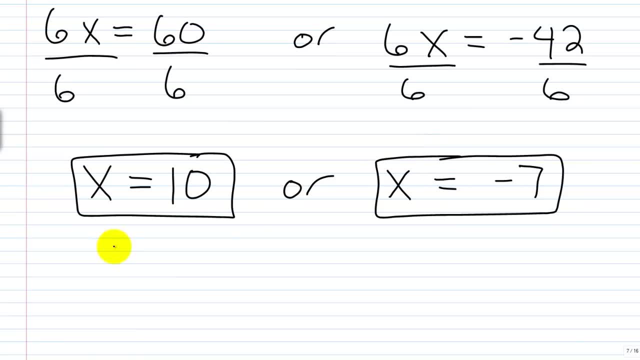 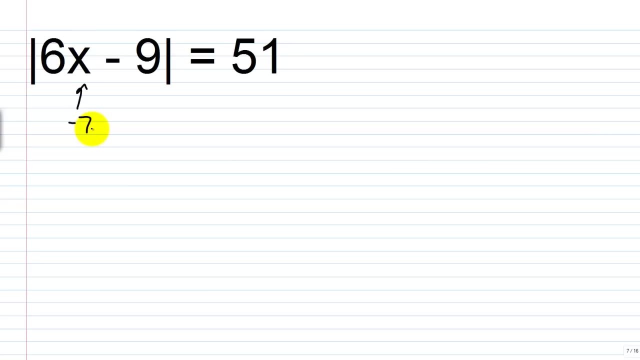 have X equals 10 or X equals negative 7. so let's write this in solution set notation. we'll put negative 7 comma 10 and let's check. let's just make sure that these work. so I'm going to plug a negative 7 in for X. let's check that one first. so 6 times negative 7 is negative. 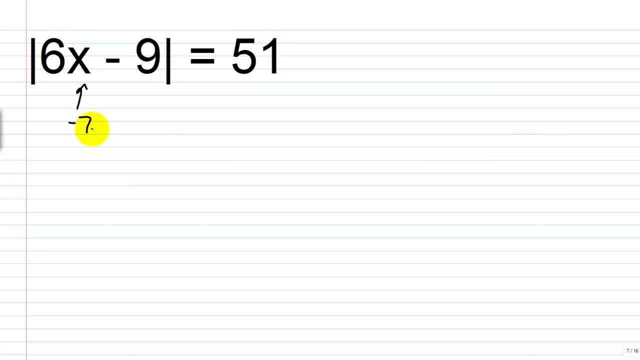 42, and then, if I subtract away 9, I'll get negative 51. so the absolute value of negative 51, as we said earlier, would be 51, right, so you'd have 51 equals 51. so that solution checks out. so now let's check 10. well, you plug a 10 in for X, you. 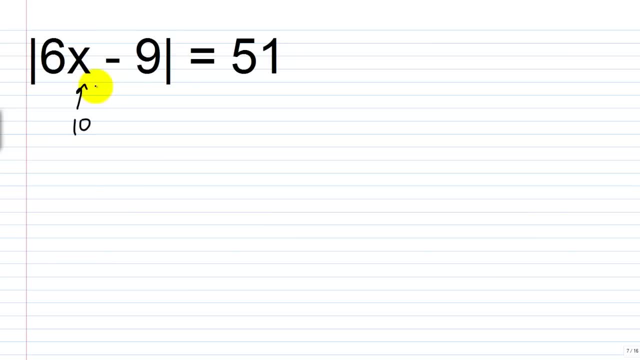 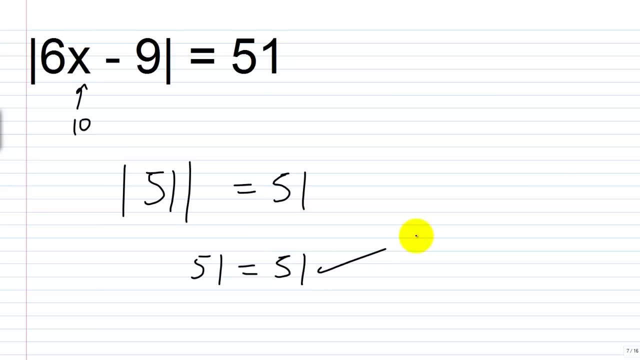 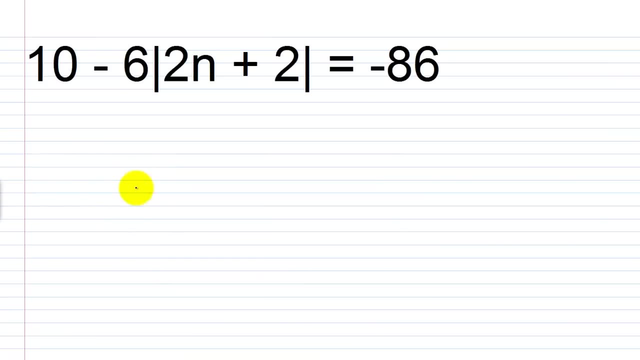 of course, that's true as well. now you get 51 equals 51, so that solution also checks out. let's take a look at a harder one, okay, so what do we do when we see something like this? we're used to seeing just something like 2n plus 2. 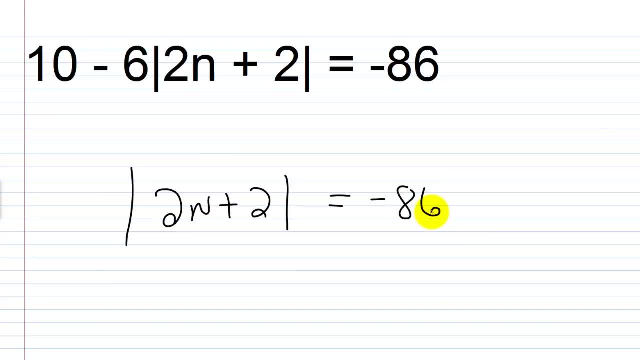 inside of absolute value bars equals negative 86, but now we've got all kinds of stuff going on outside, so we have this 10. that's subtracting away this 6 multiplied by the absolute value of 2n plus 2. well, basically what you want to. 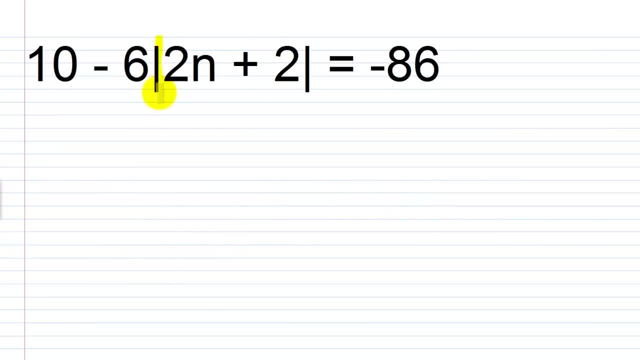 do is you want to isolate this part right here? okay, isolate the absolute value part. so the absolute value of 2n plus 2 should be on one side of the equation and the other side should be just everything else. okay, so what we're gonna do is we're gonna start by subtracting away 10 from each side of 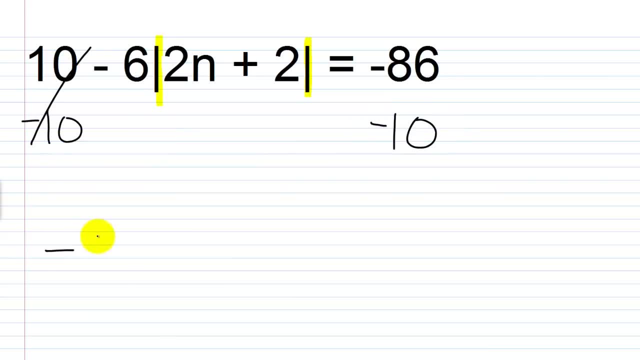 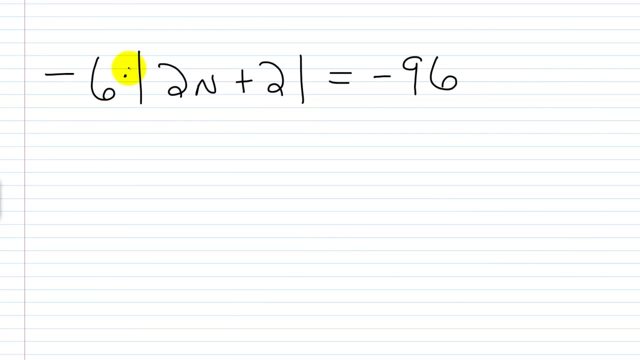 the equation. so then this will go away. I'll have negative 6 times the absolute value of 2n plus 2, and this is equal to negative 86. minus 10 is negative 96. now how can I isolate this? remember this is multiplication here. so to undo. 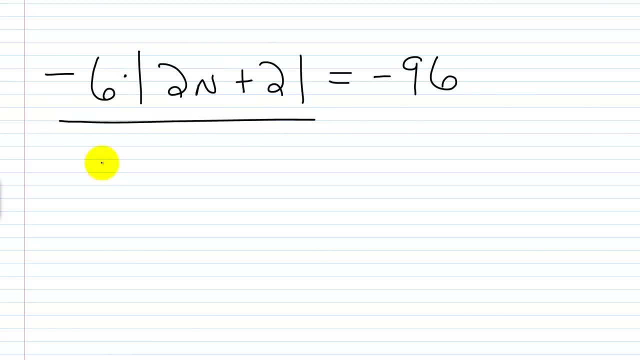 multiplication. to isolate this, I need to divide. so we'll divide each side by negative 6 and this will cancel with this and now isolated the absolute value of 2n plus 2. that's what I wanted to do. and over here, negative 96 divided by negative 6, and 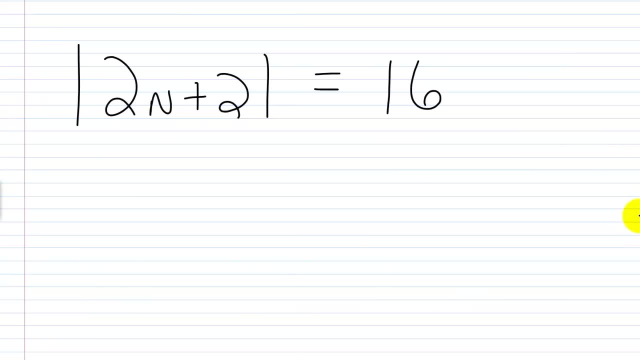 this is going to give me 16. so now this looks like something we're very familiar with. right we have the absolute value of 2n plus 2 is equal to 16, and this just sets up into 2n plus 2 equals 16. or again, 2n plus 2 could be what it could. 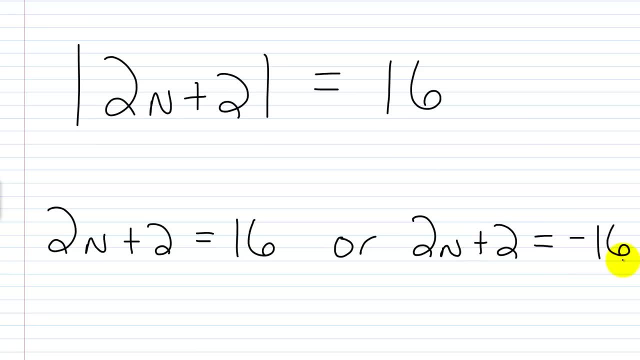 be equal to negative 16 could be equal to negative 16. kind of scroll over a little bit because again, if I plug a number in for n, I multiply it by 2, I then add 2 and the result is negative 16, which is what I'm saying right there, once I take the absolute. 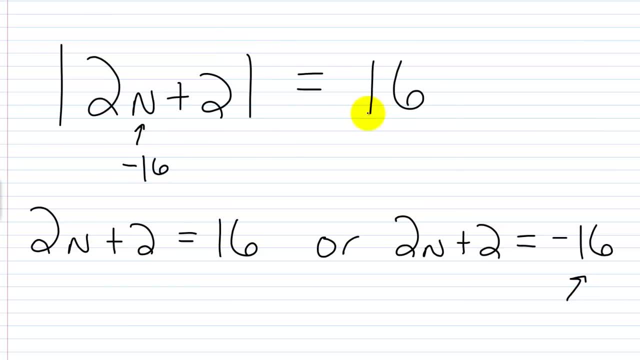 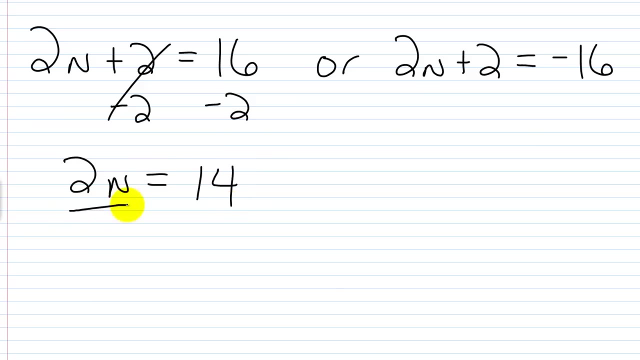 value of that, I will get 16, and that'll give me a true statement. okay, so let's solve these two simple equations over here. I'm going to subtract away 2 from each side to start, and I'll have 2n equals 14. I'll divide each side by 2 and 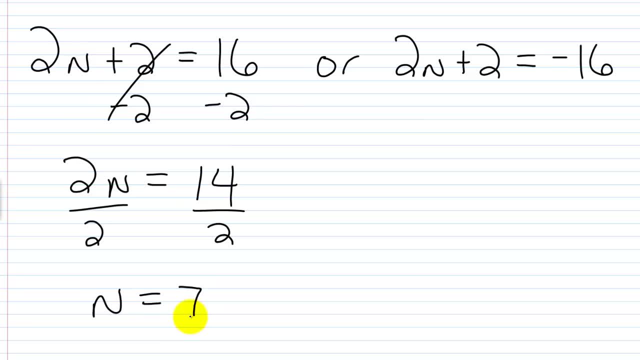 you'll get n equals 7. okay, so that's one solution over here. I'll subtract away 2 from each side. that'll cancel. you'll have 2n is equal to negative. 18. divide each side by 2 and you'll have n is equal to negative. 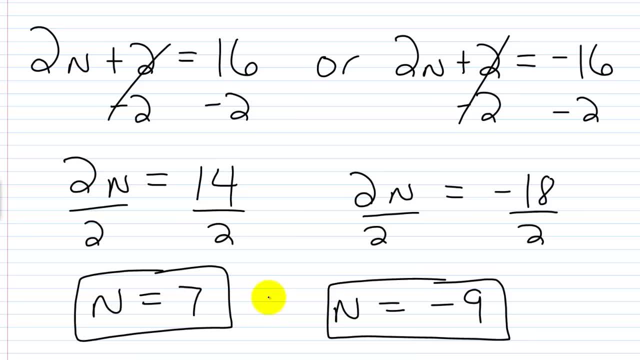 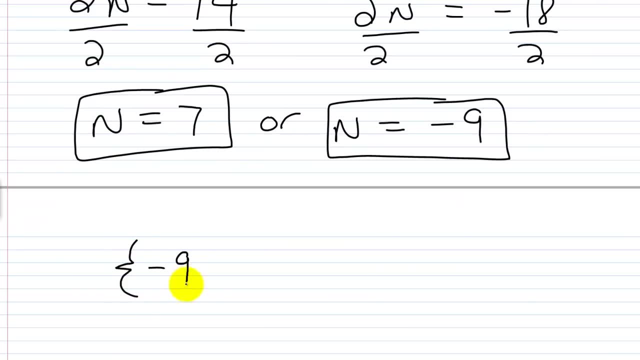 naught. so I have n equals 7 or n equals negative 9. let's write our solution set and I'll let you go ahead and plug these two back in. in other words, you'll plug a plug in a negative 9 for n in the original equation. so right there, you plug in you. 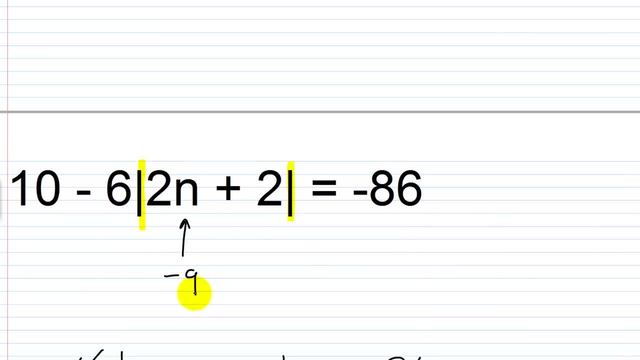 kind of erase this. you'll plug in a negative 9,, okay, and then you'll also, once you're done with that, plug in a 7.. So go ahead and do that on your own and make sure that the left and the right side are equal in value once you're done. Okay, let's take a look. 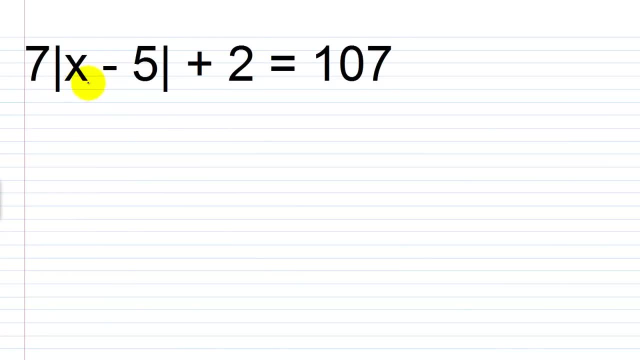 at another one, We have 7 times the absolute value of x minus 5, then plus 2, is equal to 107.. Okay, so again, we want to isolate this absolute value part. okay, isolate that absolute value part. So subtract away 2 from each side. that'll cancel. you'll have 7 times. 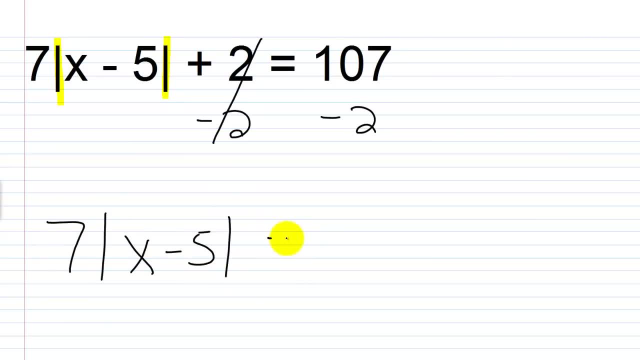 the absolute value of x minus 5, and this will be equal to 107 minus 2, is 105.. Now, because we have again multiplication here, we need to divide each side by 7.. So this will cancel over here. 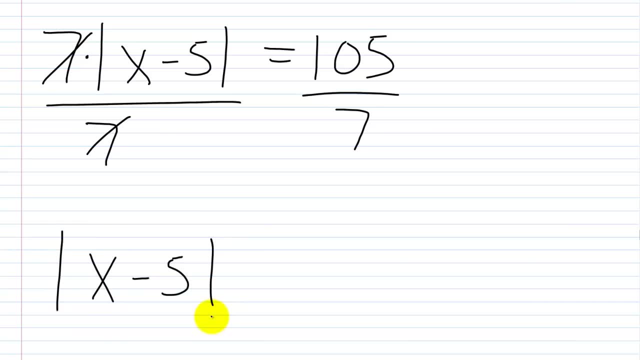 And I'll have the absolute value of x minus 5 by itself on the left. On the right, 105 divided by 7 is 15.. So now this is in a format that I know how to work with. Again, all I'm. 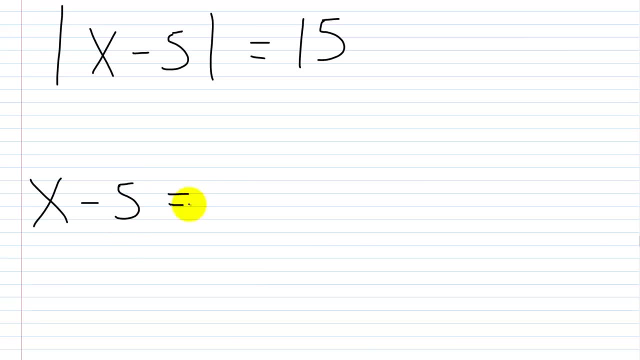 going to do is set up two simple equations: x minus 5 could be equal to what 15?? Or again, x minus 5 could be negative 15.. x minus 5 could be negative 15.. And again, why is that? 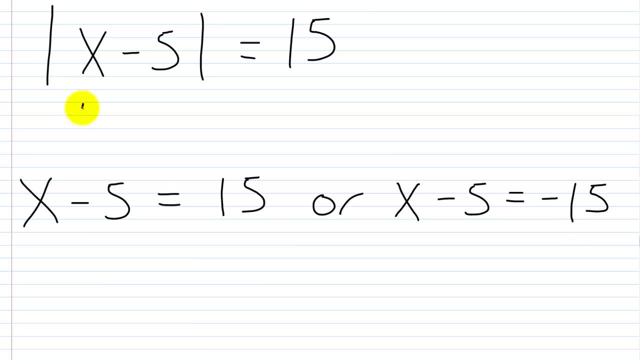 the case. Why could x minus 5 be negative 15?? Because if I plug in a value for x and I subtract away 5, and I get negative 15 as a result, once I take the absolute value it's going. 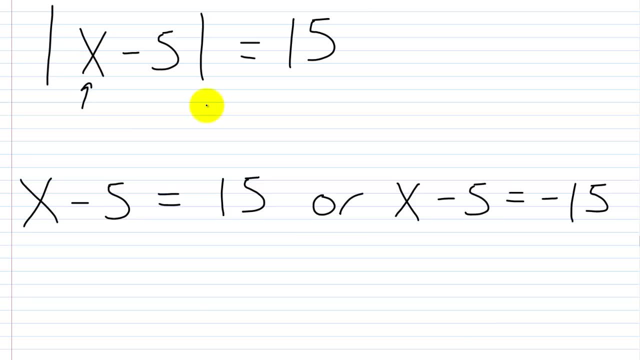 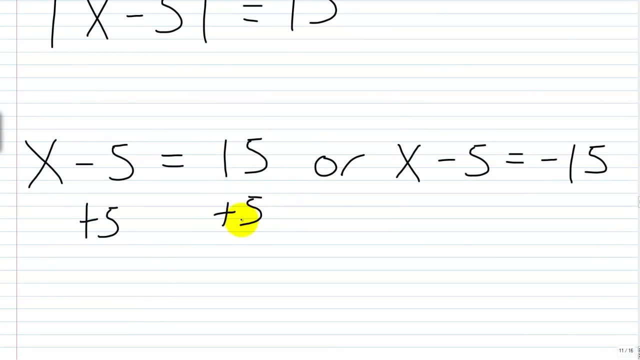 to give me 15.. So I'd have 15 equals 15, that would give me a true statement. Okay, let's solve these two simple equations and all I need to do is add 5 to both sides to get x by itself. So I'll have x equals 20. over here or over here, I'll add 5 to each side. 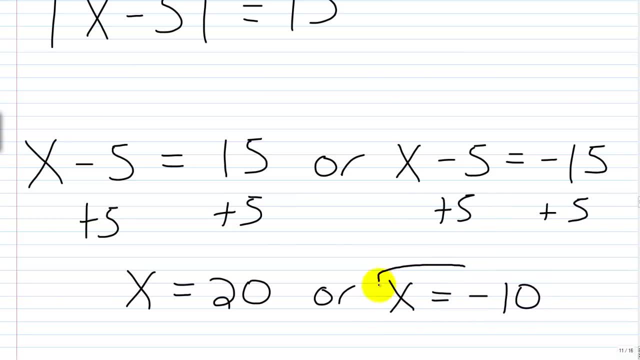 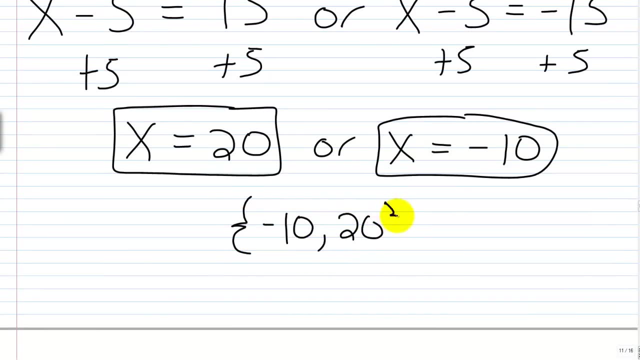 and I'll have: x equals negative 20.. So I'll take my final value and write x to the left I'm going to, and in specific here I'll add negative 10.. So those are my two solutions. Then the negative 10 gets. 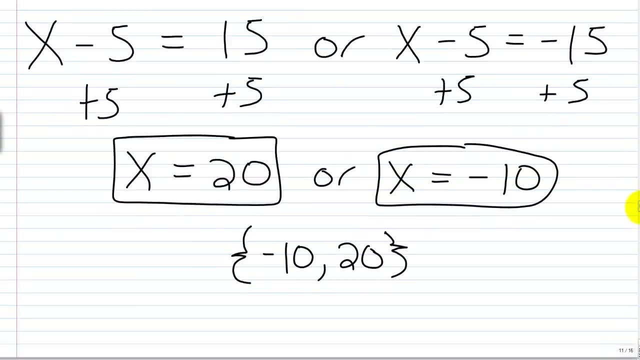 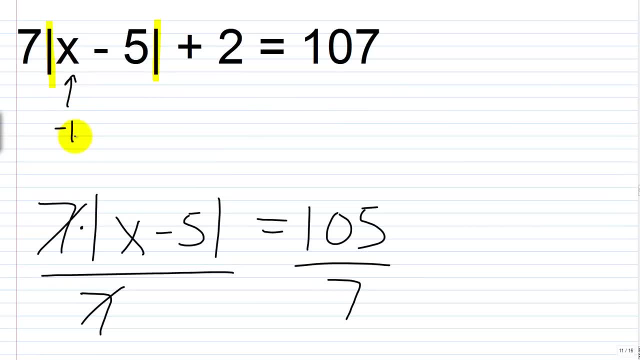 10, Juice. Okay, negative 10 comma 20 would be my solution set And then take each one. so take negative 10 and take 20, go back to the original equation, which is this one. all the way back up here You're going to plug in the negative 10, evaluate and make sure. 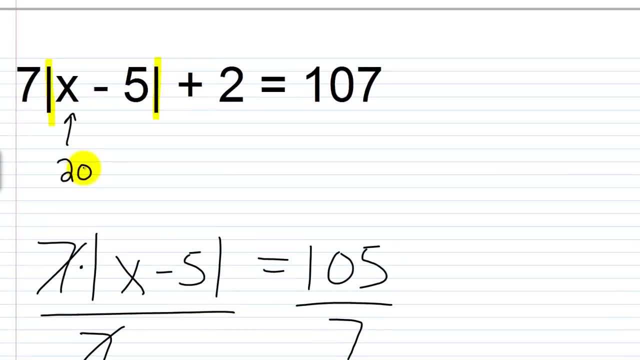 the left and the right sides are equal, Then you're going to plug in a 20. Okay, Evaluate. make sure the left and the right side that are equal- don't effort a 20. Okay, evaluate side- are equal. I'll leave that up to you to do. Okay, let's take a look at another one We have 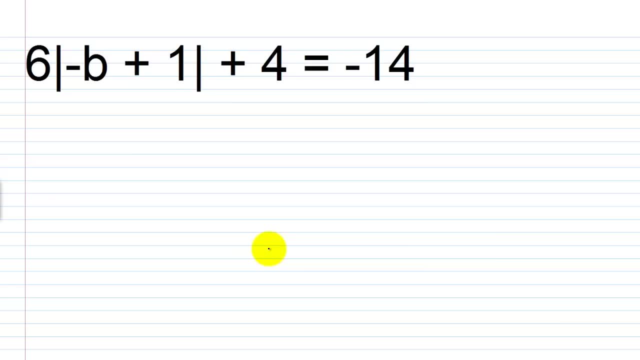 six times the absolute value of negative B plus one. then we add four to this and it's equal to negative 14.. So again, we want to start by isolating this absolute value part, this absolute value part, And what we do is we subtract away four from each side. So that's going to cancel. 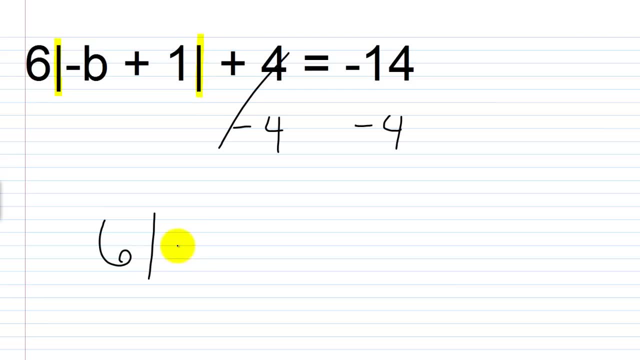 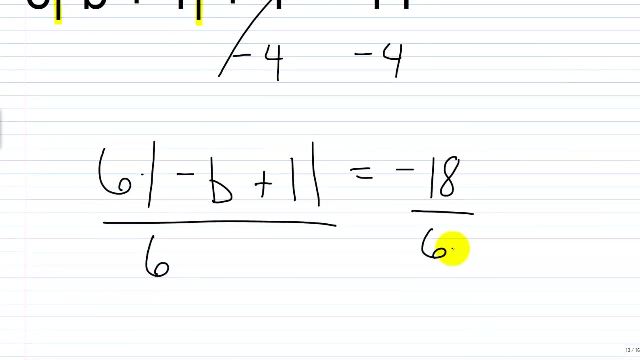 And we're going to have six times the absolute value of negative B plus one is equal to what negative 18.. And I want this by itself. Remember, this is multiplication here. So to undo that, I divide. So divide by six over here, divide by six over here. So then this cancels with this. 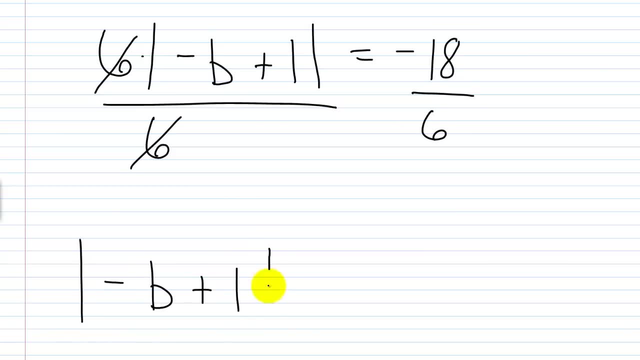 and I'll have the absolute value of negative B plus one is equal to negative 18 divided by six is negative three. Now here's where we're going to stop, And a lot of you will already know from your intuition or you've solved problems like these before you know, that we don't have a solution here. 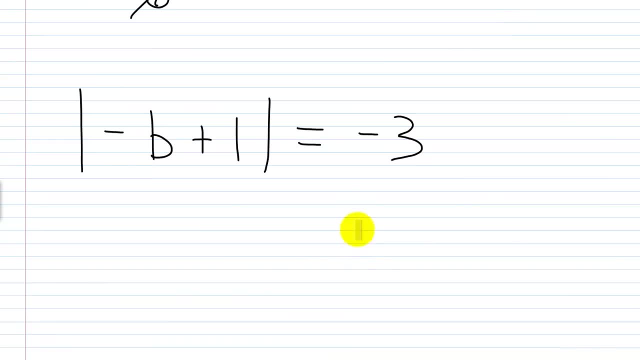 And for those of you who are confused, let me explain why. So the reason there's no solution is because this number right here is negative. We should know that the absolute value of, let's say, some number A is always going to be greater than or equal to zero. It can be anything that's zero. 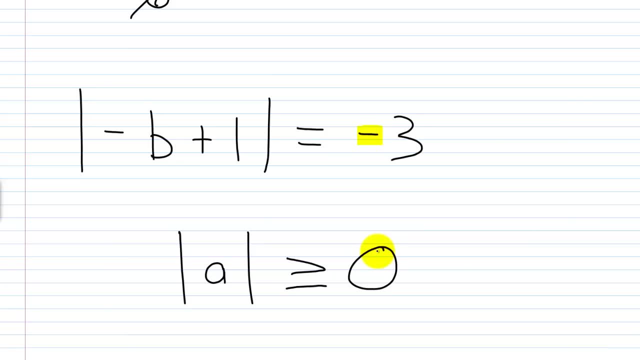 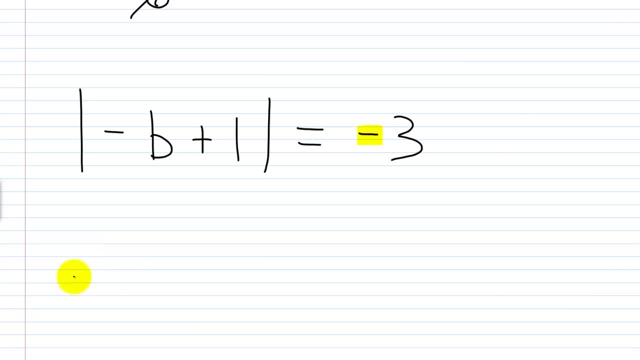 of students, I'll see they get this problem here and they just go: okay, well, negative B plus one could be equal to negative three. or negative B plus one could be equal to three. No Wrong, wrong, wrong, And you can try that out. Try solving those equations and plugging in the result. 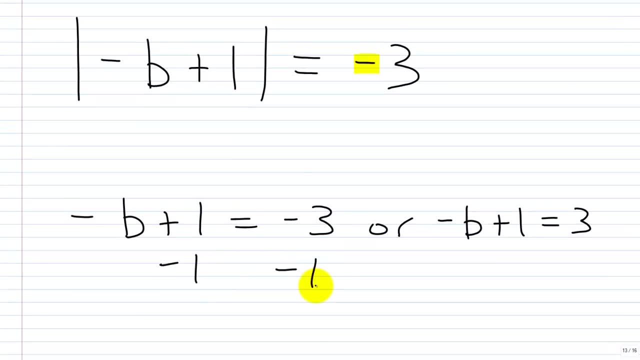 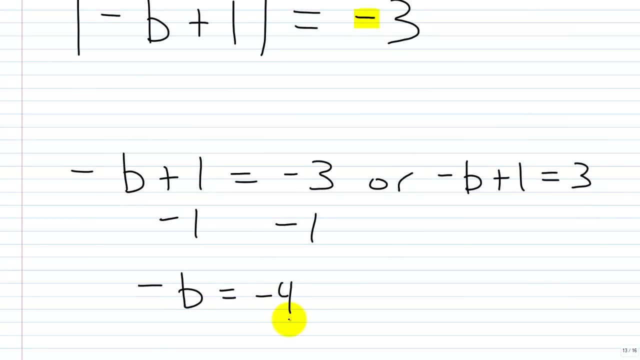 You won't get a true statement. If I subtract the way one from each side here, what would happen? I'd have negative B equals negative four. Of course B there would equal four. So go back up and plug in a four for B and see what. 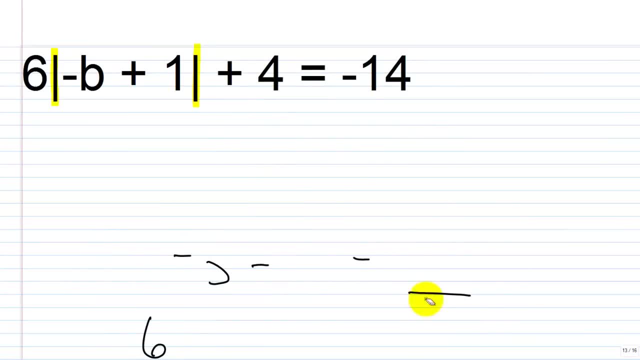 happens. Plug in a, four for B and see what happens. So you'd have negative four plus one and that would give me negative three. So you'd have basically six times the absolute value of negative three. And we know the absolute value of negative three is what It's positive. 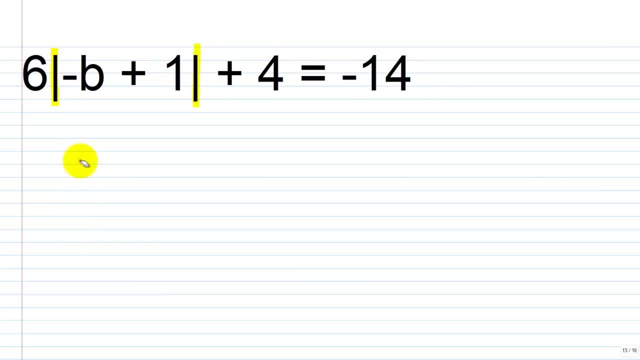 three. We've made this positive, So six times positive. three is 18. So you'd have 18 plus four, And 18 plus four is 22. So you'd have 22 equals negative 14, and that is false So. 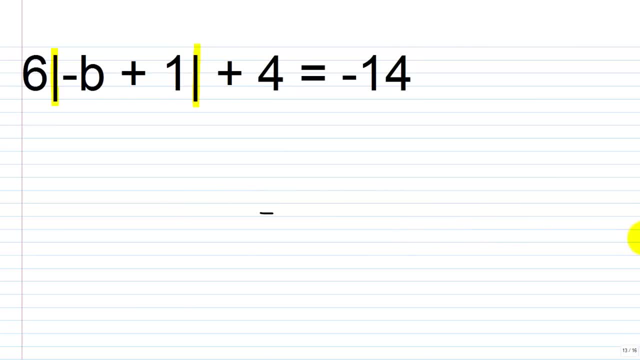 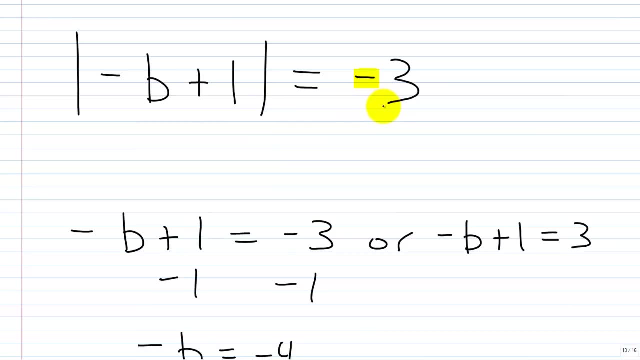 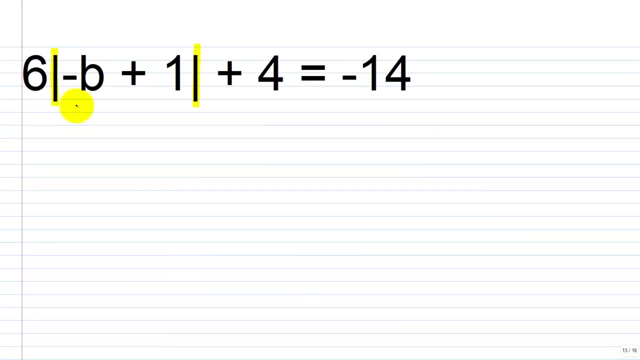 you see, that doesn't work out. Again, when you get to this step right here and you've isolated the absolute value part and it equals some negative number, you don't have a solution, And so you just write the symbol for the empty set, because your solution set contains no elements. 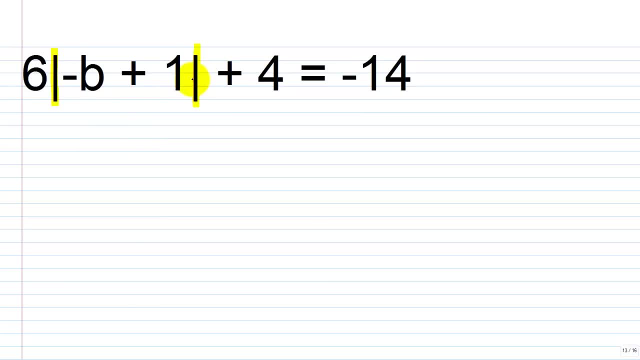 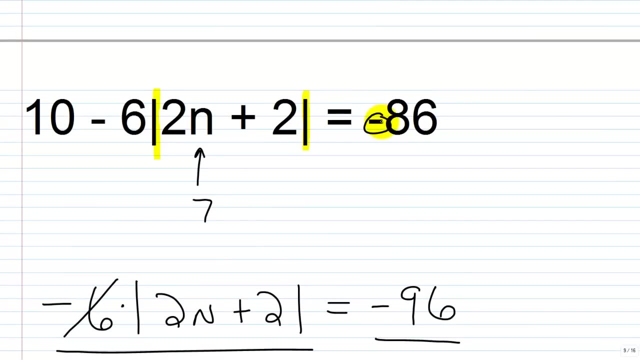 So one thing I want to tell you is make sure you actually isolate this first before you make that determination, Because remember, up here in this problem this was equal to a negative over here. So that's where a lot of students get confused as well. They'll. 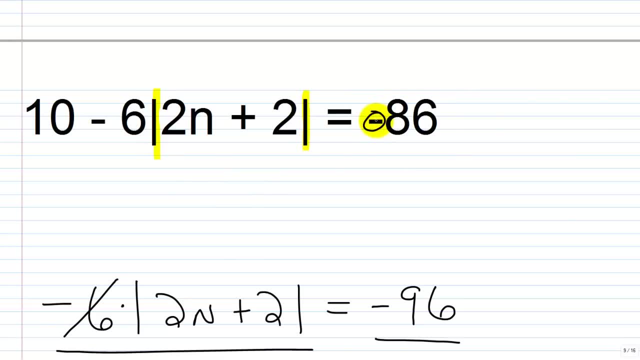 see a problem like this and go: oh, this is equal to a negative over here. So all of a sudden it's null set. They'll go boom. that's the answer. What you want to do is go through and isolate the absolute value part, So the absolute value part is equal to something. 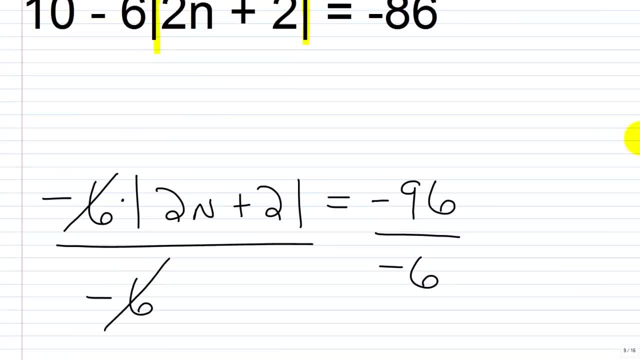 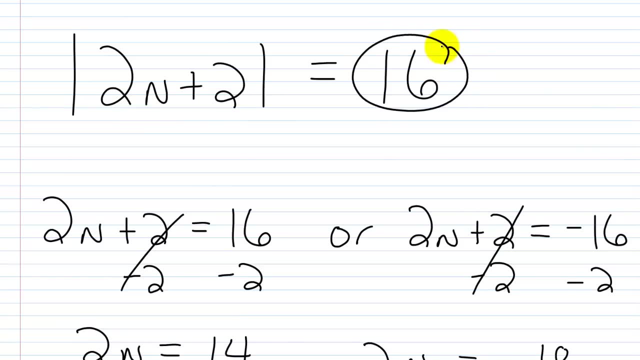 And if that something is negative, in the end you won't have an answer. Here we had an answer because we went through and we end up with this: absolute value of 2n plus 2 was equal to 16. It was positive Over here again, again, again. I can't stress this enough. 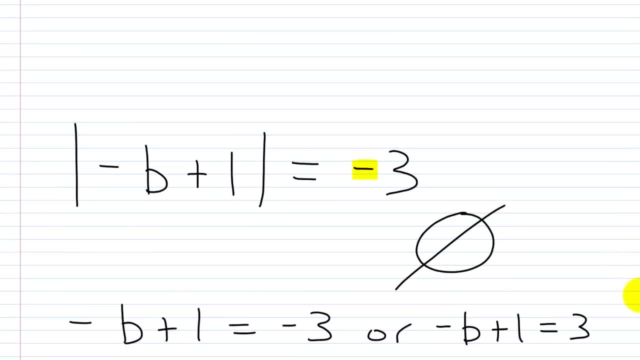 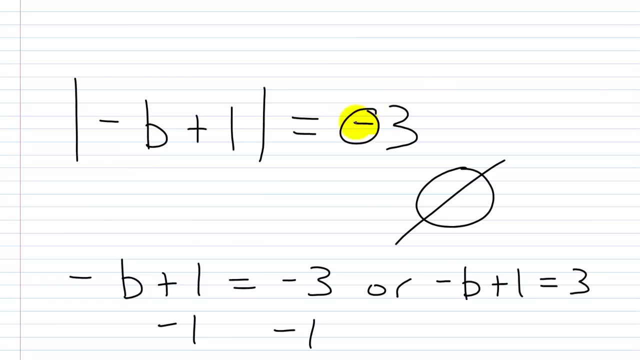 Once we did our procedure to isolate the absolute value part, we ended up with a negative over here. So the absolute value of negative b plus 1 was equal to a negative 3. And again, again, that does not have a solution. So this symbol we use for the null or empty set. 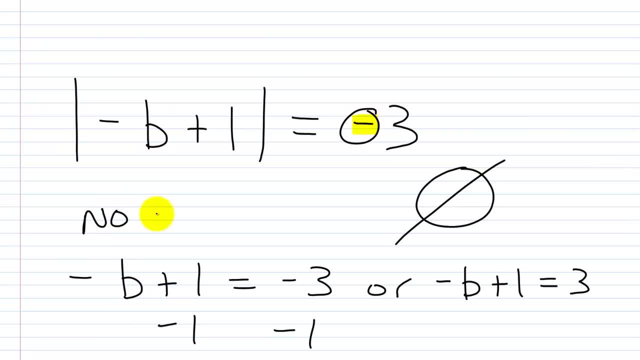 is what we would write for our answer, or some teachers would accept no solution. Okay, let's take a look at one final problem. This is another one that gives students a lot of headache. So basically you have: the absolute value of 7x plus 1 is equal to the. 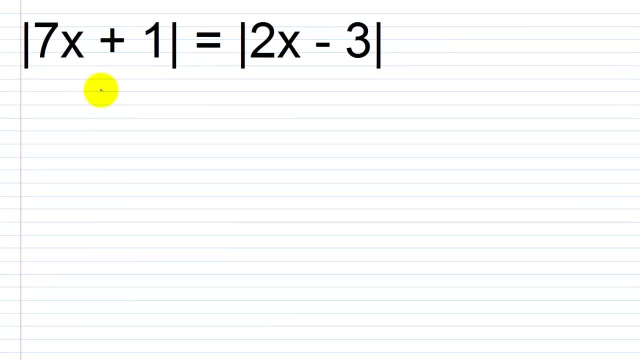 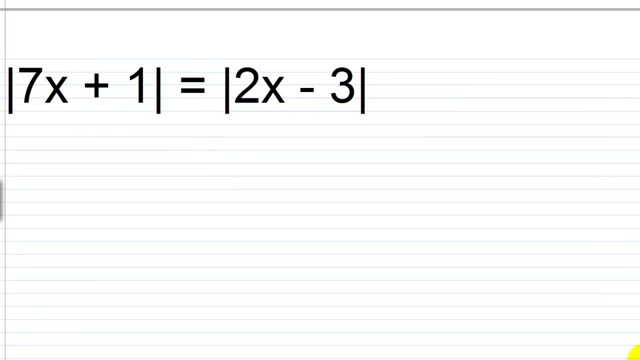 absolute value of 2x minus 3.. So how do you solve something like this? Well, basically, what you want to do is: you want to solve something like this. You want to solve something like this. What you want to do is think about what I told you in the beginning of the lesson. 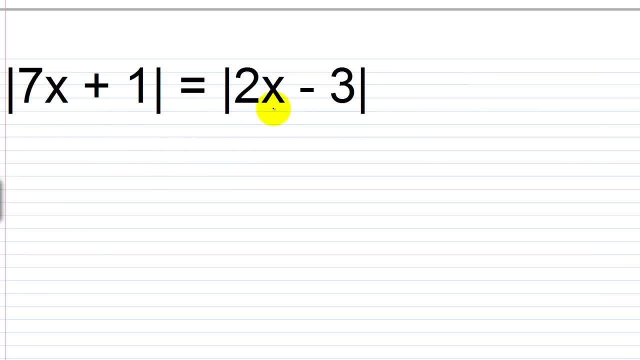 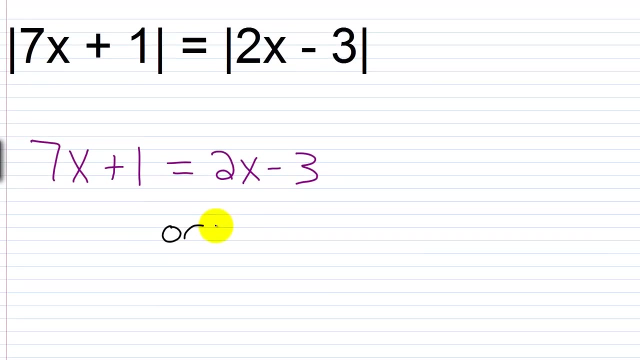 So basically, these two expressions can only have the same absolute value if they're equal. So meaning 7x plus 1 is equal to 2x minus 3.. That's one solution, Or another possibility is that they're opposites or negatives of each other. So 7x plus 1 would be equal to. 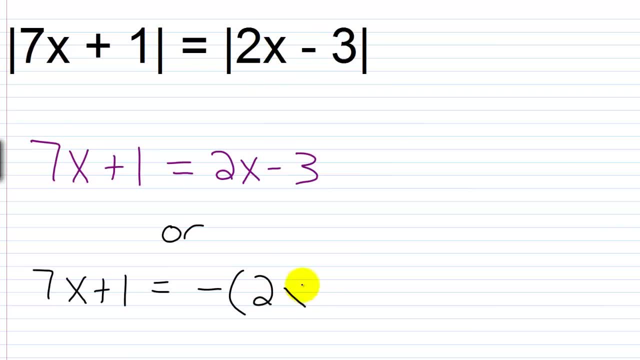 the negative of this whole thing: 7x plus 1 is equal to 2x minus 3.. Make sure you use parentheses. Don't make a silly mistake like this. Right, Then you're just making the 2x part negative and you're not changing. 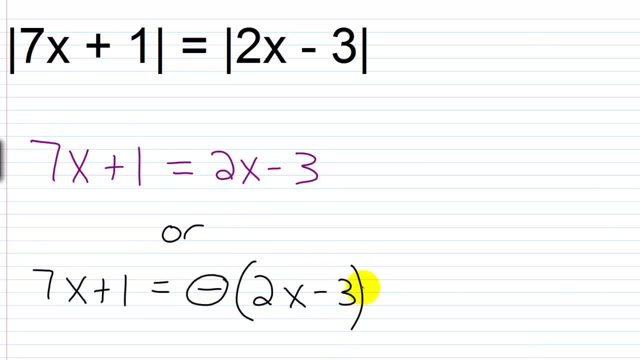 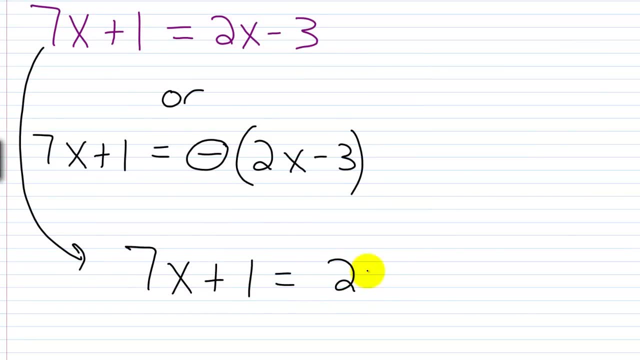 this to positive. Got to put parentheses because it's the opposite of this whole expression: 2x minus 3.. Let's start with this one: 7x plus 1 equals 2x minus 3.. And pretty easy to solve this. 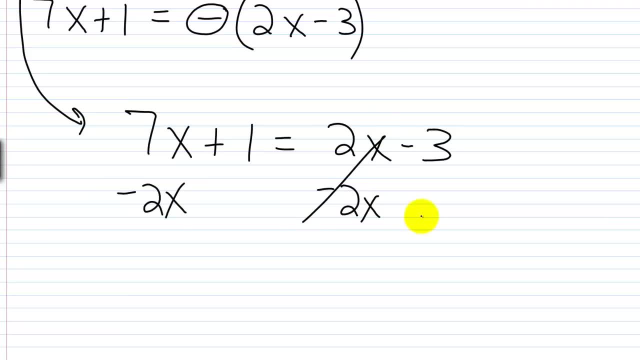 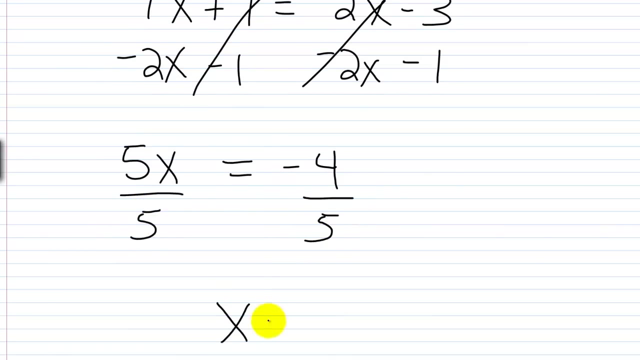 Just subtract away 2x from each side, That's gone. You'll have 5x over here, And then you'll subtract away one from each side, That's gone. We'll have negative 3 minus 1 is negative 4.. Just divide each side by 5.. You'll have x equals negative 4 fifths. So there's one. 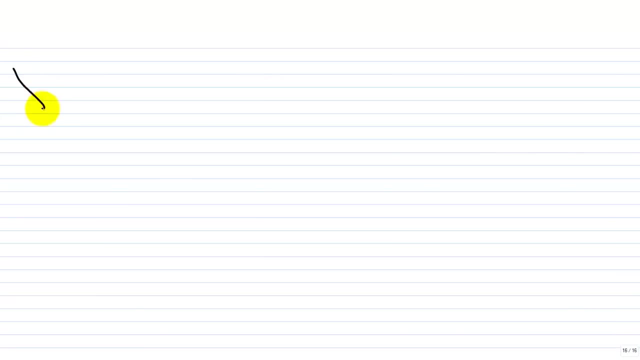 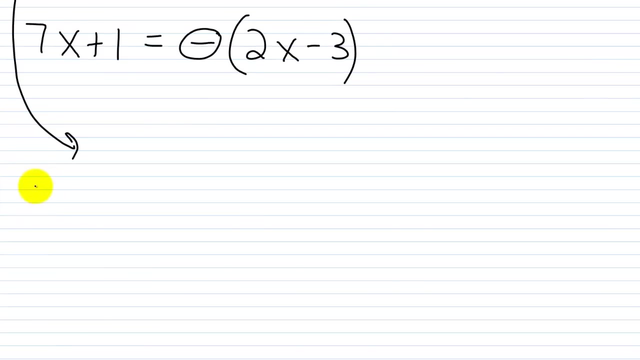 solution. Let me just scroll down and get a little room here. I'll write that down here: X equals negative 4 fifths, And let's do the other one now. So we have: 7x plus 1 is equal to the negative of this. so just distribute the negative negative times: 2x is negative 2x and 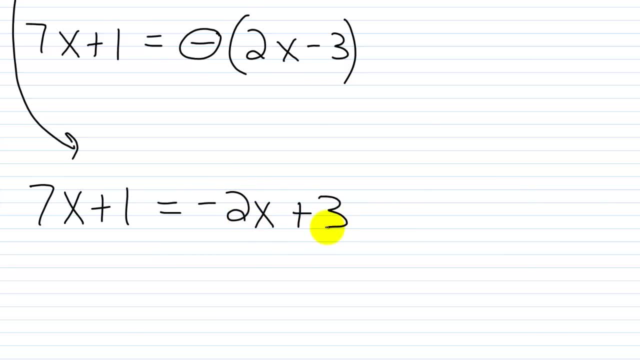 negative times: negative 3 is just plus 3, and we solve it the same way. let's just add 2x to each side, that's gone. let's subtract 1 from each side, that's gone. so 7x plus 2x is now 9x and 3 minus 1. 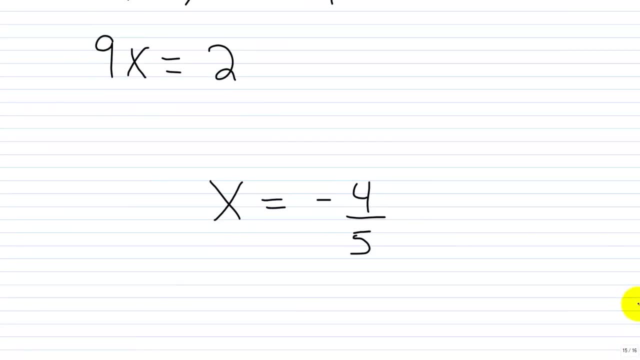 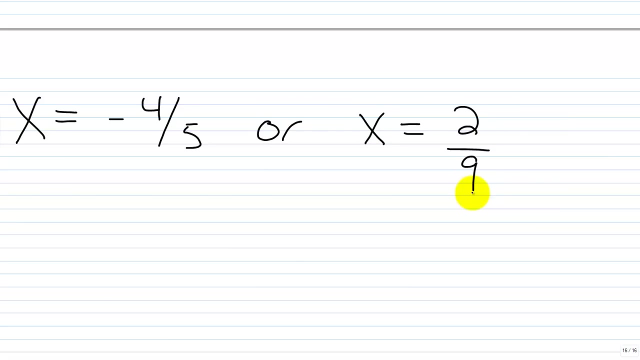 is 2, so we'll divide each side by 9. we'll get x equals 2- 9ths as our other solution. so we have x equals negative 4- 5ths or x equals 2- 9ths. let's write this in solution: set notation: negative 4. 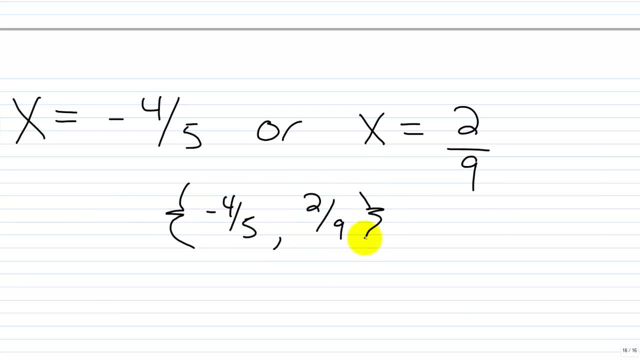 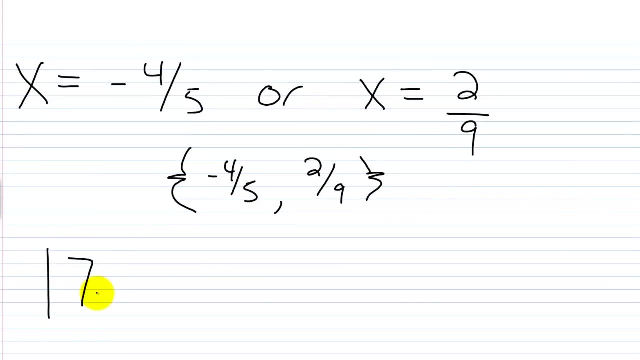 5ths, comma 2. 9ths, let's write this original equation again. again, it was the, the. The absolute value of 7x plus 1 is equal to the absolute value of 2x minus 3.. Let's start by plugging this in this negative 4. fifths. 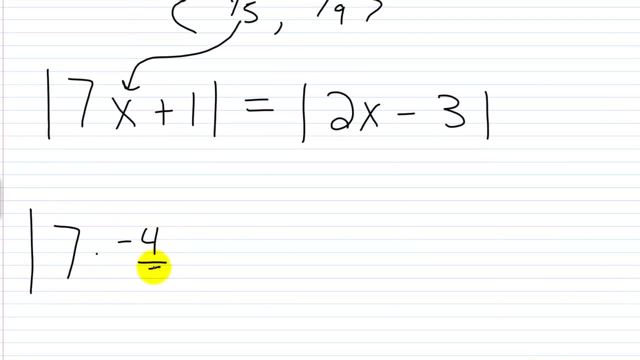 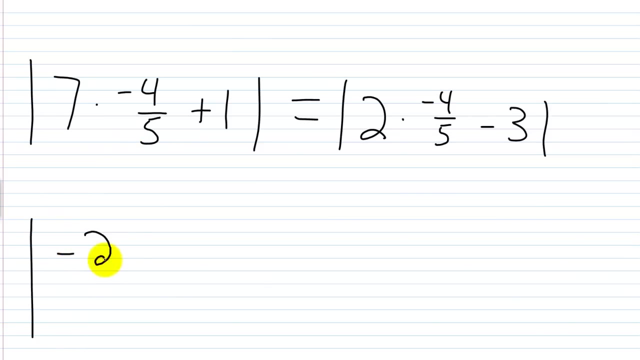 What do we get? Well, the absolute value of 7 times negative 4 fifths plus 1 is equal to the absolute value of 2 times negative 4 fifths minus 3.. So 7 times negative 4 is negative 28,. so you'd have negative 28 fifths plus 1.. 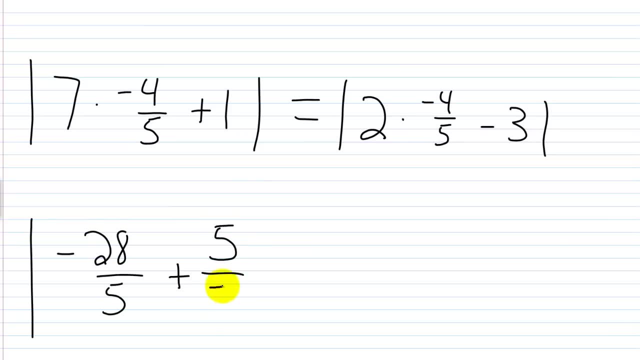 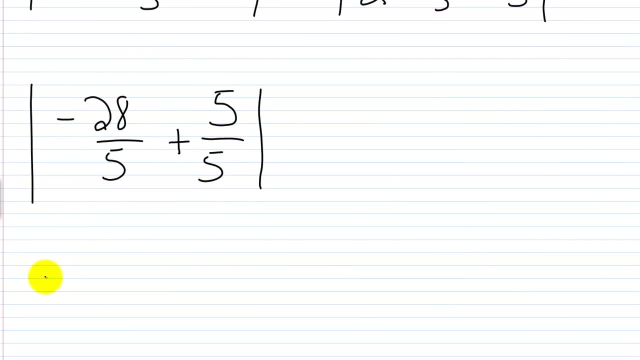 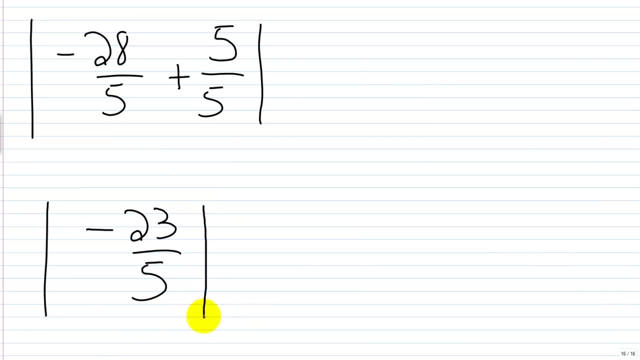 So to get a common denominator, I could just say this is 5 over 5.. Let's just kind of continue that. So basically, negative 28 plus 5 is negative 23,. so you'd have the absolute value of negative 23 over 5.. 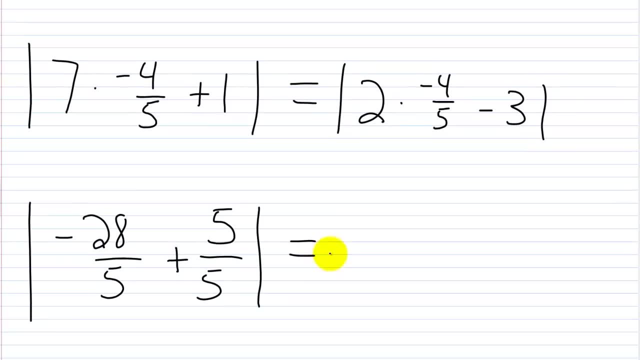 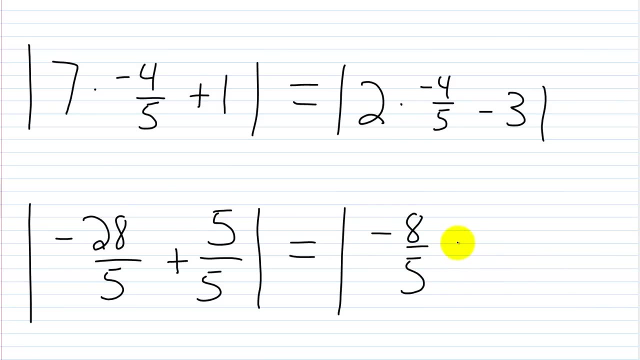 That would be on the left side. Okay, Let's do the right side real quick. 2 times negative. 4 is negative 8, so you'd have negative 8 fifths there minus 3.. To get a common denominator, you can write 3 as what. 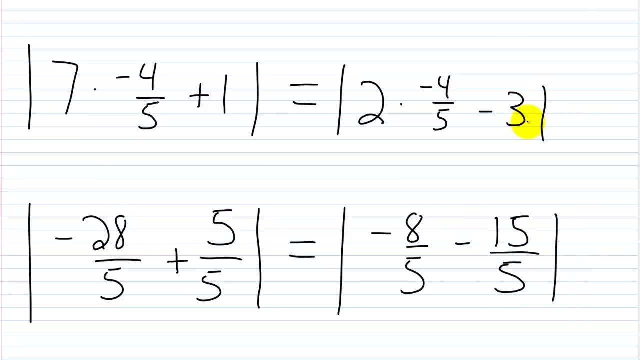 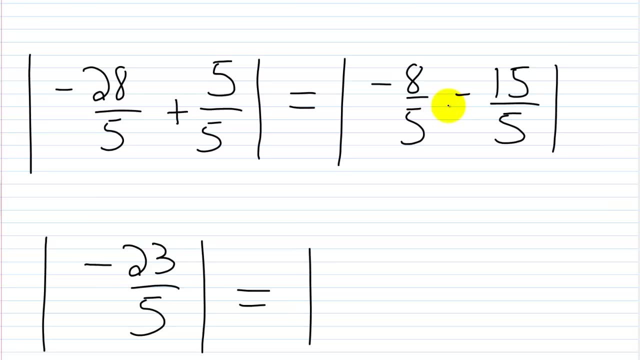 15 fifths. All I did was just multiply this by 5 over 5.. Okay, So then equals: absolute value of negative 8 minus 15 is negative 23.. So, negative 23 fifths. When you take the final step of taking the absolute value of negative 8 minus 15, you.